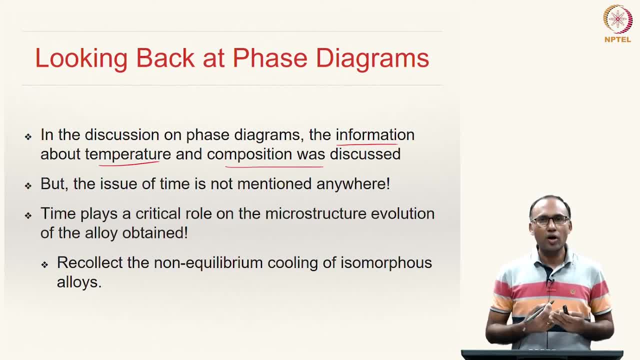 liquid phase to a solid state and at each and every instances, how long should I wait at a given temperature in order for the transformation to complete? So the issue of time is not discussed anywhere during the discussion on phase diagrams. However, time plays a critical role in the 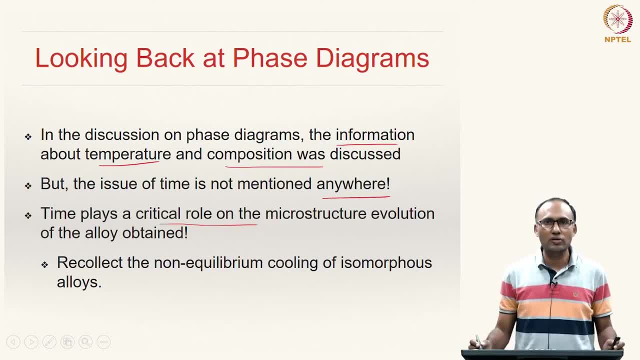 microstructure, evolution of the alloy, of any composition that we are looking at, for instance, in a binary phase diagrams, and we have actually had a discussion on the effect of time for one specific case, when we have discussed the non equilibrium cooling of isomorphous alloys. 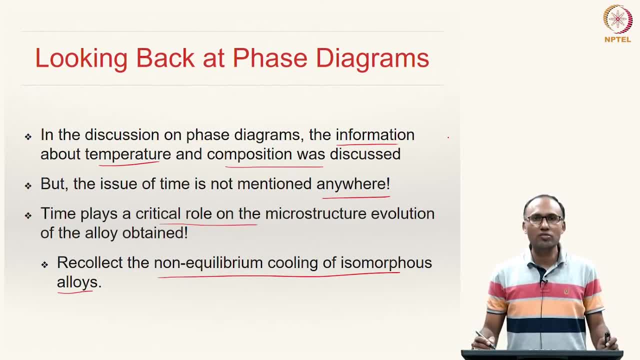 where we have shown that the microstructure that is developed during non equilibrium cooling of an isomorphous alloy is different from the microstructure obtained through equilibrium cooling. So the major difference between equilibrium cooling and non equilibrium cooling is the time involved, or that amount of time that one is that we are providing for the 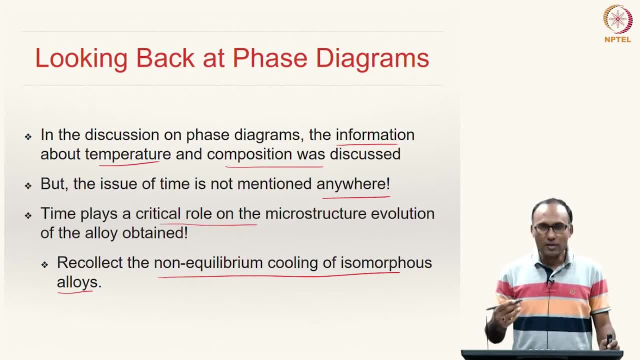 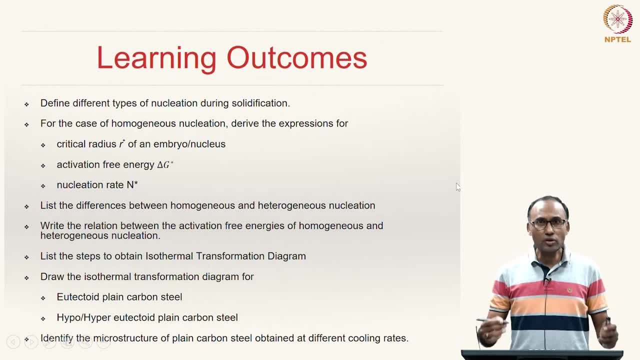 system to cool down at a given temperature right, And hence the time is the time that plays a key for the real microstructure evolution during the solidification. So in this module we will pay attention to this aspect of time and then understand how. 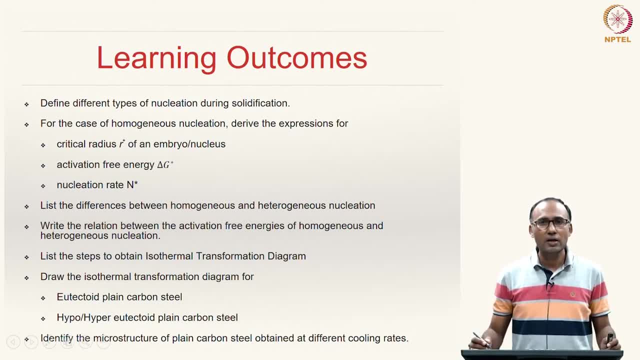 the microstructure evolution is going to get affected because of the time that is involved during the transformation. So the learning outcomes of this module, or so first we will discuss about the fundamentals of this microstructure evolution, So the microstructure evolution from the model which we have discussed earlier, which we have discussed earlier, we have discussed 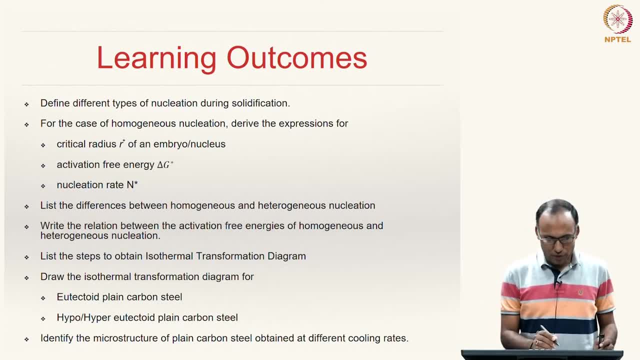 liquid state to solid state is governed by the two phenomena- one of the important phenomena called nucleation, and followed by growth. So we need to understand different types of nucleation during solidification, So we should be able to define different types of. 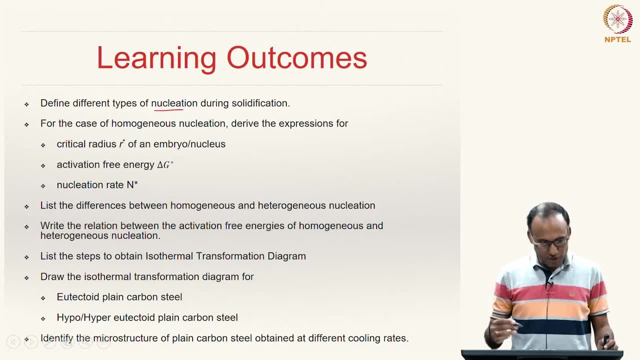 nucleation during solidification. So for the case of homogeneous nucleation we will be deriving the expression for critical radius r star of a nucleus or embryo and activation, free energy delta g star and the nucleation rate n dot. It is not n star, it is n dot. 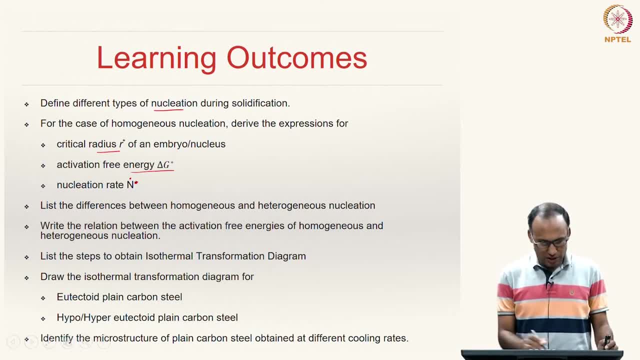 And we should have…. at the end of this module, we should be able to list the differences between homogeneous nucleation and heterogeneous nucleation right, And also we should be able to write the relation between the activation free energies of homogeneous nucleation and. 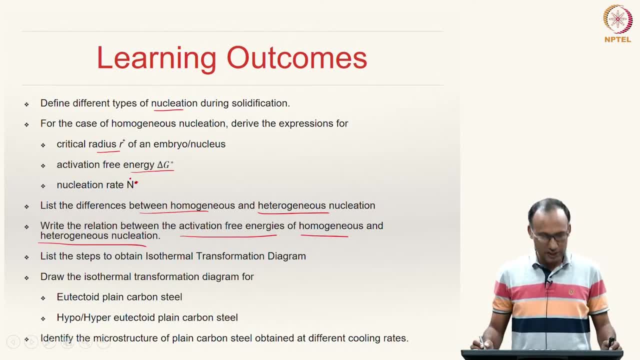 heterogeneous nucleation, how their activation free energies are related, And then we will talk about an important concept called isothermal transformation diagram, And then, when we…. while we are talking about isothermal transformation diagram, we should be able to list various experimental steps that one needs to undertake in order 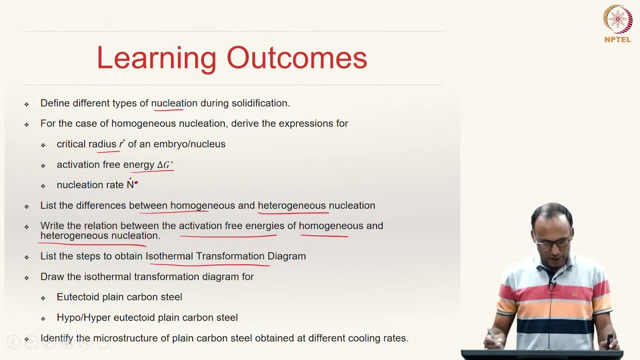 to generate such an isothermal transformation diagram And we should be able to draw the isothermal transformation diagram for eutectoid plain carbon steel and hypo and hyper eutectoid plain carbon steels. Identify the microstructure of plain carbon steel obtained at different cooling rates. 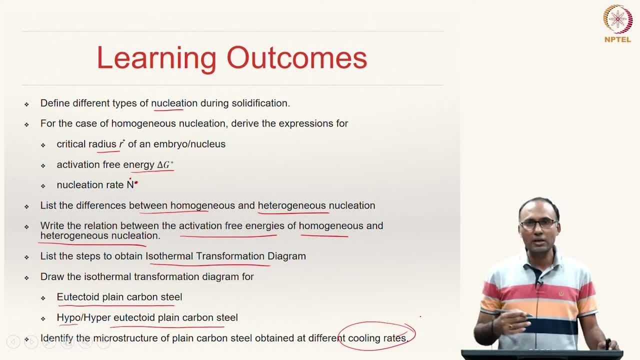 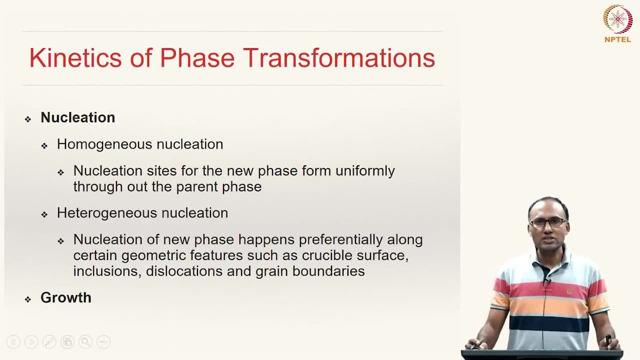 That is the key. So the time is coming here, And then we will be able to see, when we have different cooling rates, how the microstructure is evolving. So, to begin with, we will study about this. kinetics of phase transformation, So what? 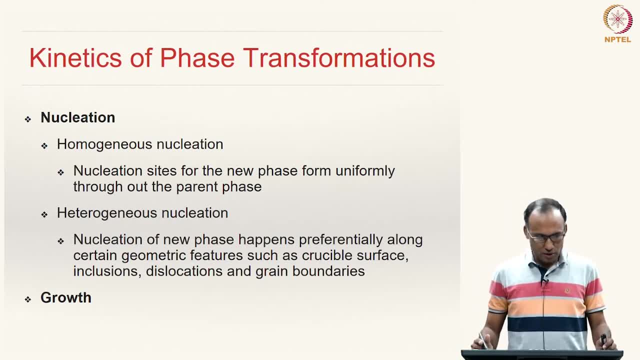 are the…. when we are talking about phase transformation, which actually essentially means two aspects. The first, you should have nucleation of the proton. The second, you should have nucleation of the product phase, So you have a liquid phase, to let us say, solid phase transformation. So this liquid phase is called parent phase. 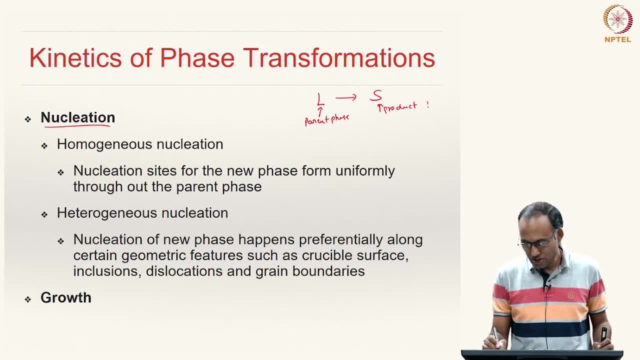 and solid phase is called product phase If your phase transformation is happening from liquid state to solid state. But, as we have seen in the discussion on phase diagrams, we also have seen transformations- phase transformations- happening within the solid state, For instance, eutectoid reaction and peritectoid reaction. These are…. 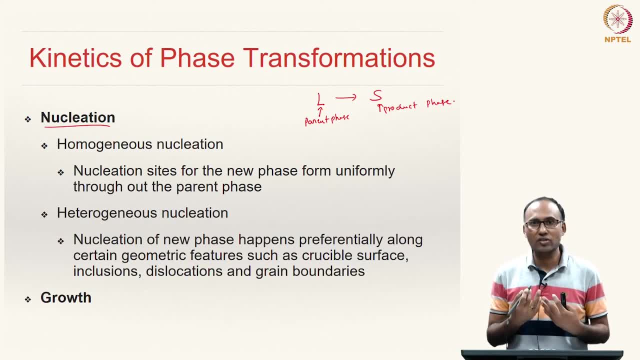 We will оously need to re- соб useful features and be sure that that歌 is something which you have not considered here. Yeah, yeah. So what are the phases? Phase transformation never happens from a liquid to solid, but it can also happen within. solid state right? So if it is—and happening from solid state 1 to solid state 2, then this is what is called our parent phase and this is our product phase. So when we are having the transformation from a parent phase to sort of product phase during eighty וה interest, 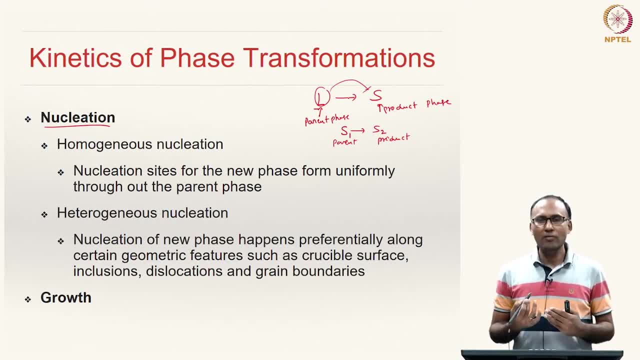 to the-in fenderiyet phase, were known to be there over half a 8 time, but for days, during eight, during this transformation, at an appropriate temperature, you have the nucleation of the product phase system. So right, for instance, whenever, whenever we are solidifying a liquid, 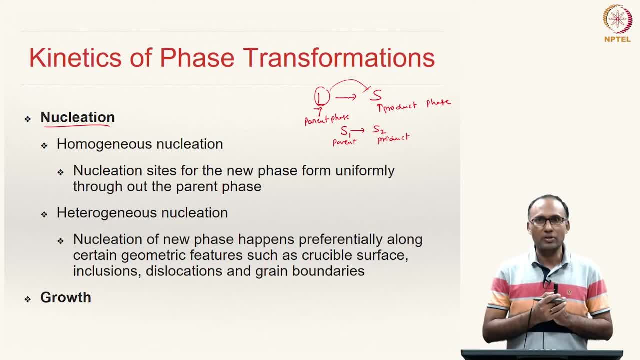 the nuclei of solid should form at the freezing temperature or solidification temperature, right? So when we are talking about nucleation, there are two kinds of nucleation. first one is homogeneous nucleation and heterogeneous nucleation. So what do we mean by homogeneous nucleation? So if the nucleation sites for the new phase 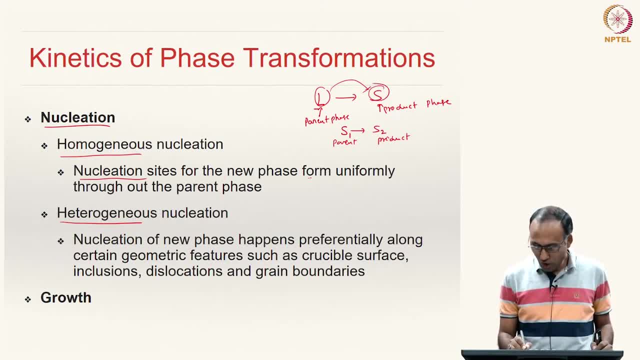 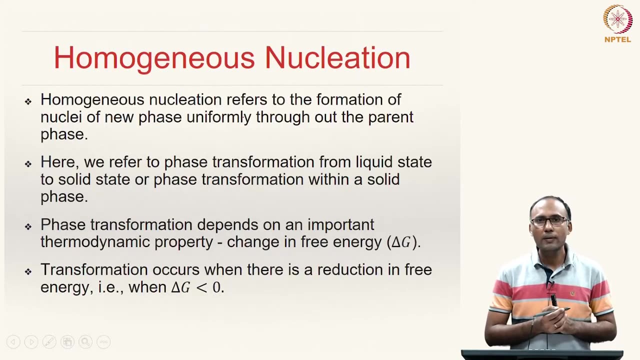 that are, let us say, in this case solid phase- form uniformly throughout the parent phase. that means, if you have say, let us say, this is our liquid, here the nucleation of the solid phase should happen uniformly throughout the parent phase. So then such a nucleation 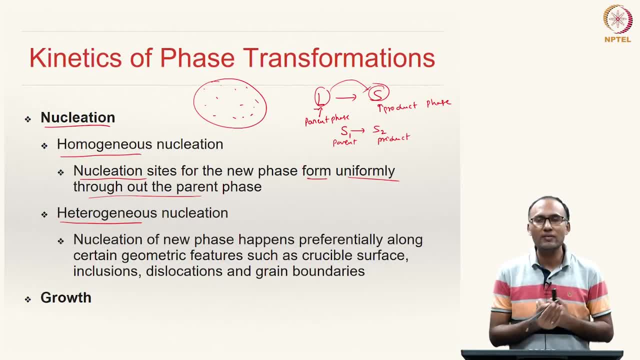 one is called homogeneous nucleation. that means there should not be any preference for the nucleation, preference of any site. there should not be any preferential sites for beginning of the nucleation. such a nucleation is called homogeneous nucleation. Heterogeneous nucleation is nothing but the nucleation of new phase happens preferentially. 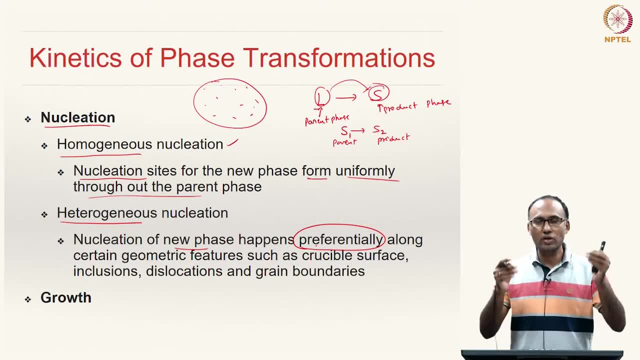 along certain geometric features, such as, for instance, if you are solidifying a liquid metal in a crucible, So the crucible surface may be one of the favorable positions where nucleation can begin right or some. sometimes you may have inclusions, So inclusion surfaces can be a favorable nucleation. 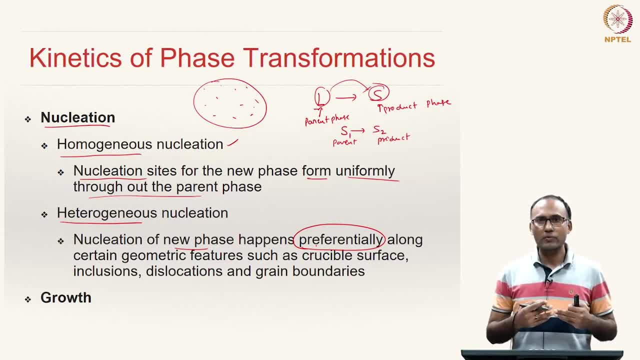 sites and similarly if you are dealing with, if you have a system where you have certain amount of liquid has already transformed to solid and already there may be some dislocations and grain boundaries that are generated. they can also be states of heterogeneous nucleation. So in a solid state, if you have transformation from one solid state to another solid state, 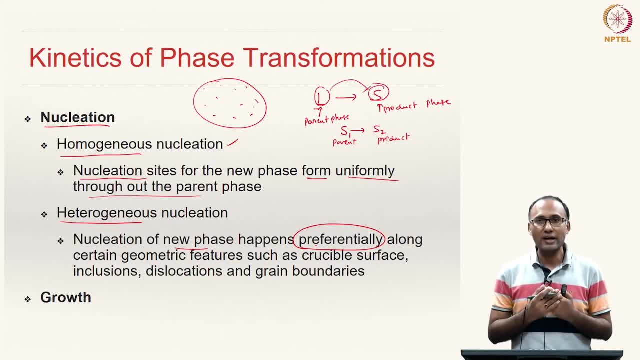 the grain, boundaries and dislocations can act as preferential sites for nucleation. So in principle you can have these two kinds of nucleations- homogeneous and heterogeneous nucleation- and once the nucleation of a product phase begins, then this nucleus has to grow in order to finish the complete transformation. So the next stage is growth stage right. 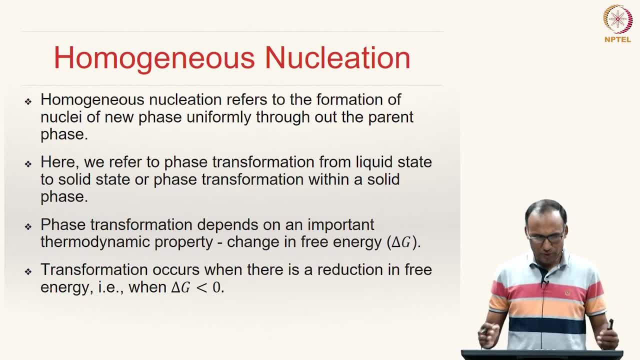 All right. So now let us try to understand, or spend some time understanding, homogeneous nucleation and derive certain important expressions that we have discussed in the learning outcomes. So, as we have already mentioned, the homogeneous nucleation refers to the formation of nuclei. 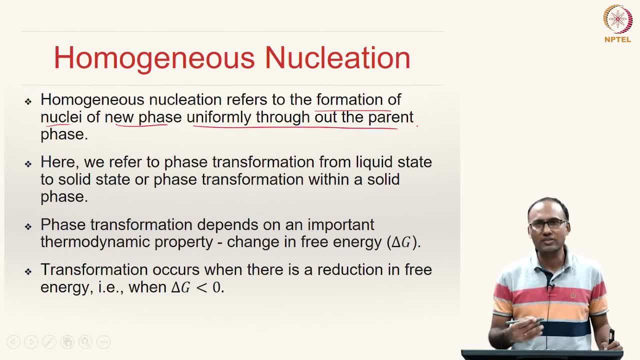 of new phase or product phase uniformly throughout the parent phase. So there is no preference whatsoever for the location where the nuclei has to form. So for instance, here we are going to use the equal to gs minus gl. that should be less than 0. So always your phase transformation happens. 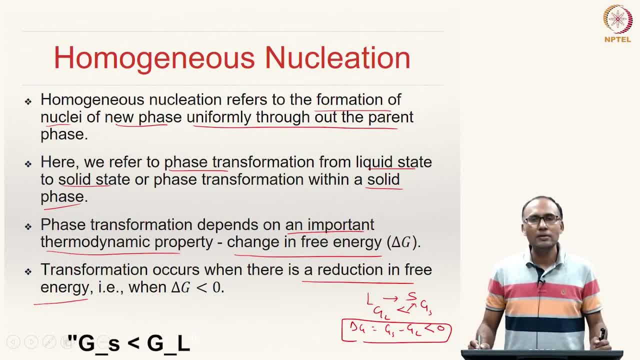 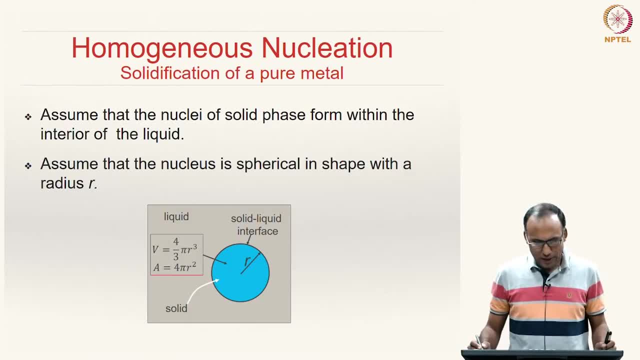 from one state, one phase, to another phase, only when the change in free energy is negative. okay, So now let us try to look at the solidification of a pure metal under homogeneous nucleation. So assume that this grey area that I am showing, 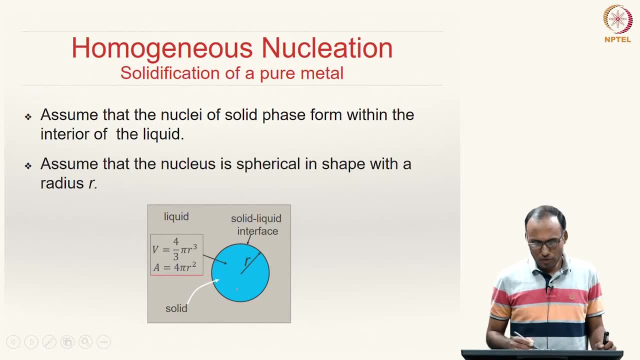 here is our liquid right. So now let us assume that the nuclei of solid phase one. we are paying attention to one nucleus, but there are several such nuclei formed uniformly throughout the liquid phase, because it is homogeneous nucleation, but we are paying attention to one such nuclei. Assume that the nuclei of solid phase form within the 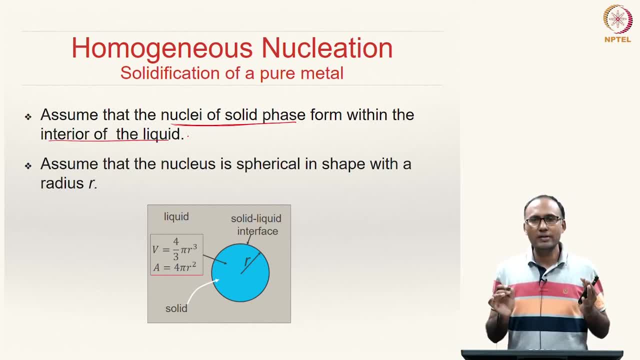 interior of the liquid. So if we have a liquid pool, you are assuming that the solid phase is nucleus is forming within the interior- It is not forming on the boundary- and we are assuming that the solid phase is the nucleus is having a spherical shape. that is an assumption, but the methodology that we are developing 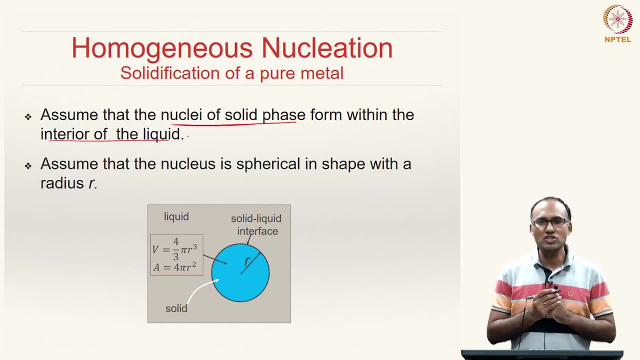 can be applied to any other shape too. but to make the discussion simple, we are going to assume the nucleus to be of spherical shape, So the assume that the nucleus is spherical shape with a radius r. So as shown in here, the blue colour, this is our nucleus, or solid. 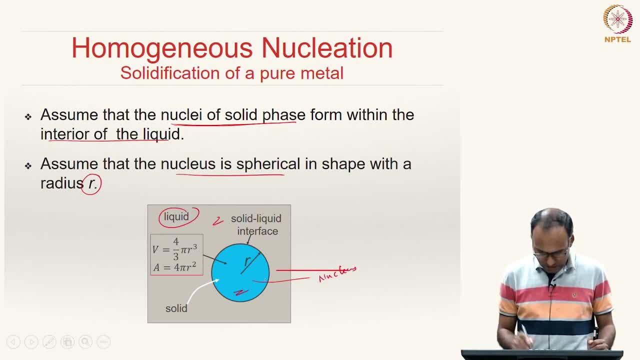 Okay, So this is our liquid. the grey colour region and this blue colour region is solid nucleus. and then this line, the boundary, the circumference of this circle. So it is shown in 2D, but it is a sphere, okay, and this is the solid liquid interface. And if you have a solid 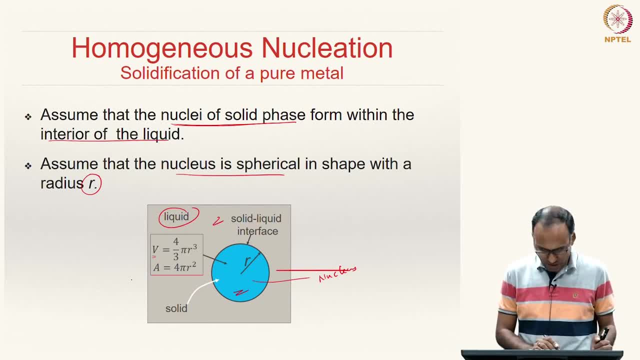 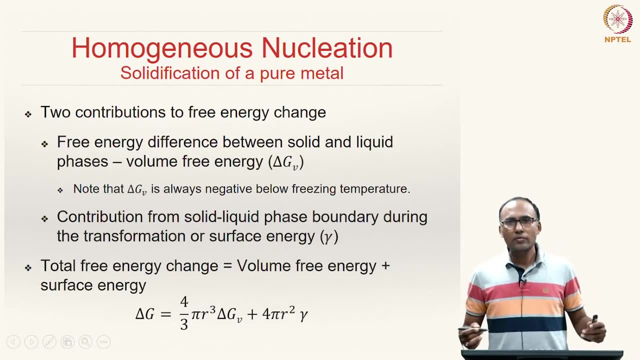 of sphere of radius r, then the volume of this sphere is 4 third pi r cube and the surface area is a pi a is equal to 4 pi r square. alright, So now, when we have, So we have a system like that, there will be two contributions to free energy change. 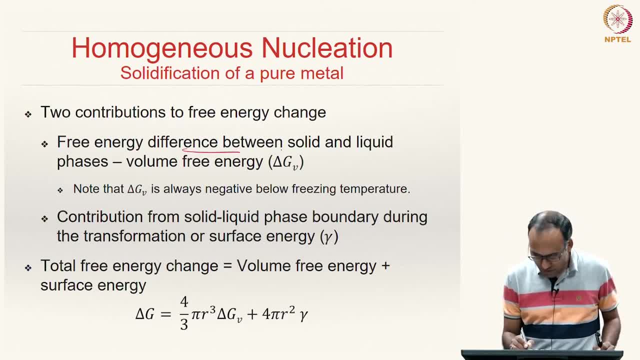 First contribution is the free energy difference between solid and liquid phases. right, The free energy difference between solid and liquid phases, which is not, which is going to be negative? then that is what we are calling volume free energy. So delta g v is called volume free. 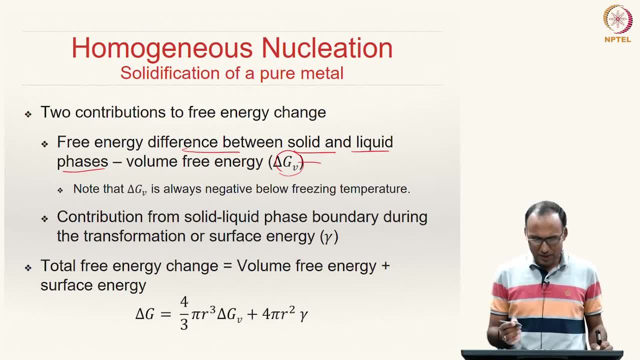 energy, which is negative if at all. the phase transformation is happening because the solid, the difference between the free energy, between the solid and the liquid phase, has to be So solid. phase free energy should be less than the liquid phase free energy. So the free. 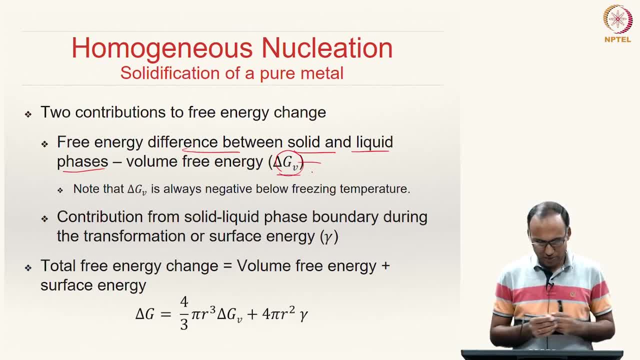 energy difference between solid and liquid phases is called volume free energy represented by delta, g, v, right. So the contribution from solid liquid phase: boundary again. So there is. there should be another. one contribution is from the volume. another contribution is coming from the boundary or surface during the transformation. that is called volume free. 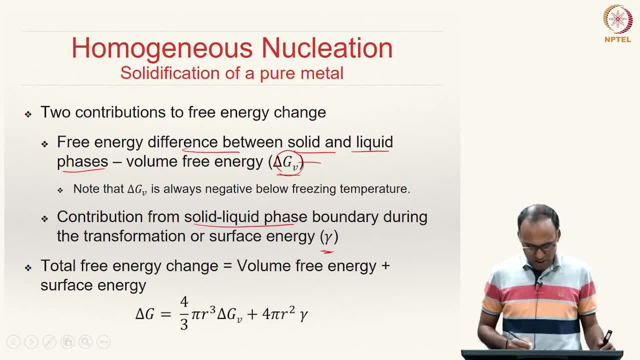 energy, surface energy. So the total free energy change is equal to volume free energy plus surface energy. So the volume free energy is nothing but volume times free energy change. So that is 4. third pi r cube is the volume of this sphere and free energy change or volume. 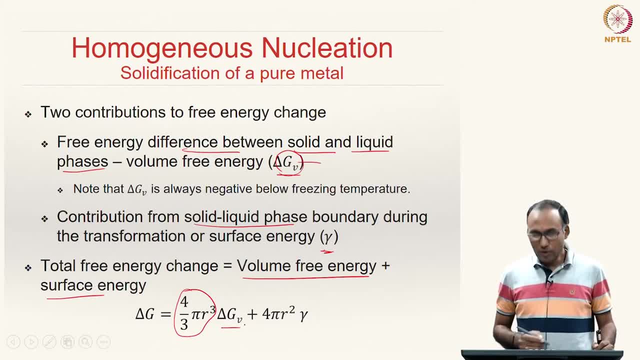 free energy is delta g v And your surface energy change is actually 4 pi r square, because before that there is no surface, now you have, So surface energy. So surface energy and gamma is the sorry 4 pi r square is the surface area and gamma is the surface energy. 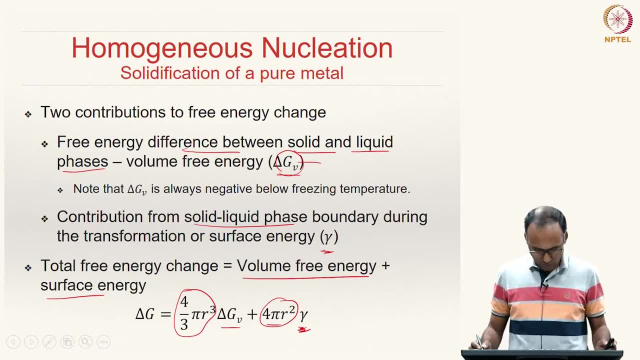 associated with the interface boundary between solid and liquid. So this is the total free energy change, delta G represented by delta G. So now, if you would plot the two quantities, that is, volume free energy and surface energy, and the total quantity, note that this is a negative quantity and this is positive quantity. 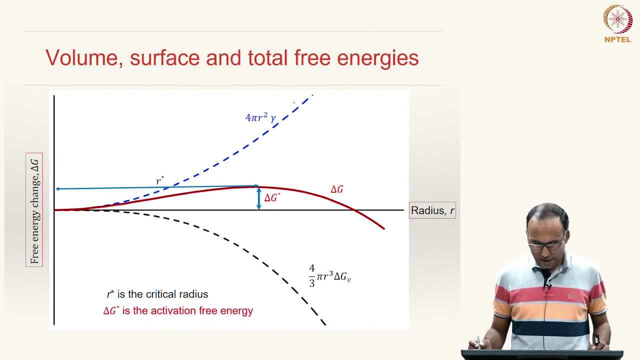 So you can see that this blue dash line is our surface energy term, So 4 pi r, square gamma, and the black dash line is our free energy volume, free energy term. and now the sum of these two is described by this red line, red solid line, which actually shows: 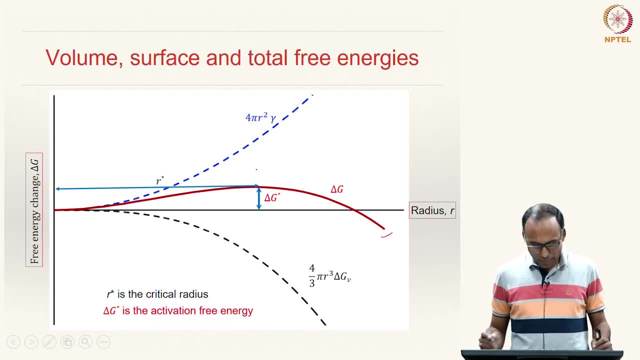 a maximum and then decreases, right So the maximum value of delta G. after which what is happening? So up to here, the free energy is increasing, Right, And then it is decreasing. However, here please note that this free energy, total delta G is: 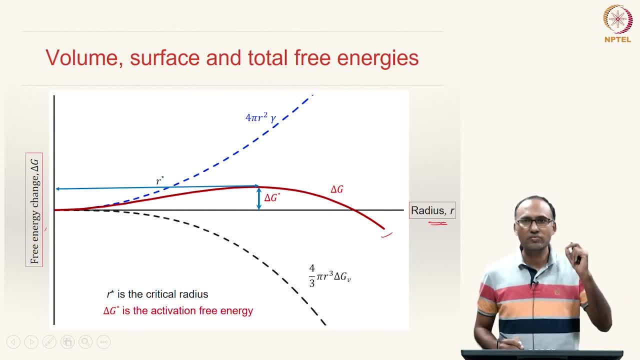 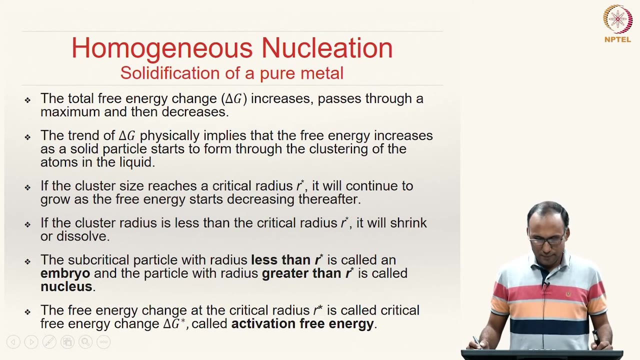 plotted as a function of radius of the particle or radius of the nucleus. So you have a free energy change as a certain feature, which is increasing first and then decreasing. Let us try to understand what is the meaning of that. So we see that the total free energy 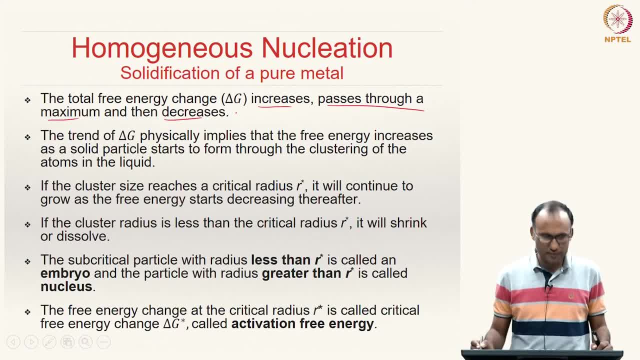 change increases, passes through a maximum and then decreases. So this trend of delta G physically implies that the free energy increases as a solid particle starts to form through the clustering of the atoms in the liquid. So what happens when the solid particle is starting to form? the atoms form, the liquid state should be coming together and to be. 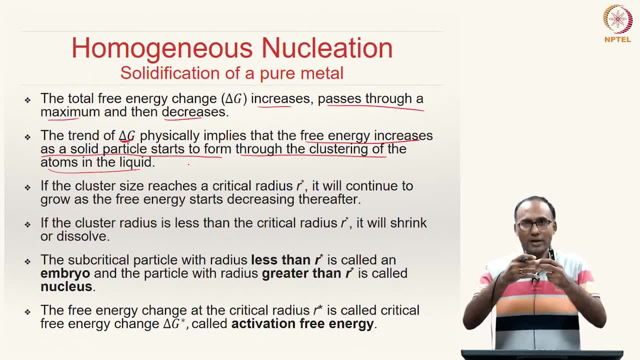 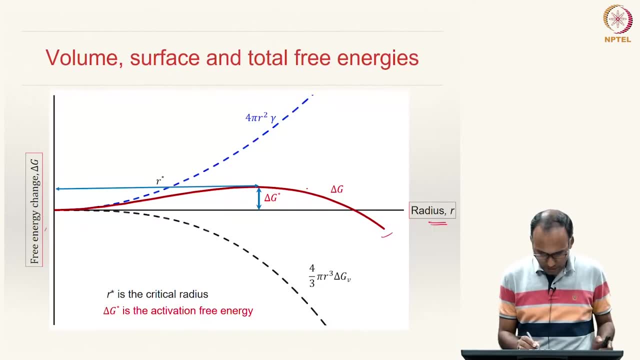 clustering to form a nucleus right. So when such a process is happening, the free energy change, the delta G is first increasing and then decreases. So this is what we are describing here. So delta G will be in the. So if the cluster size reaches a critical radius r star, as we have seen here, if the 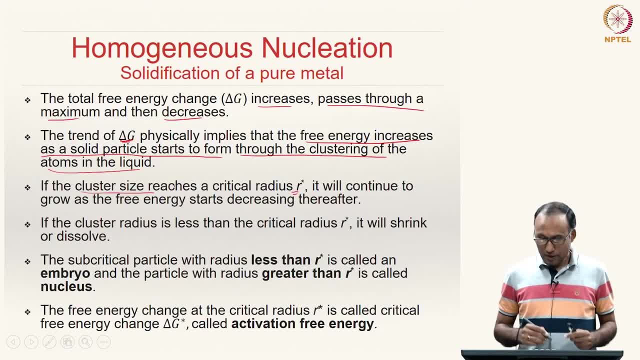 cluster size is this distance r star, it will continue the nucleus So that will continue to grow as the free energy now starts decreasing thereafter. So if the nucleus size becomes equal to r star, so the clustering of atoms of liquid state to form solid state from the 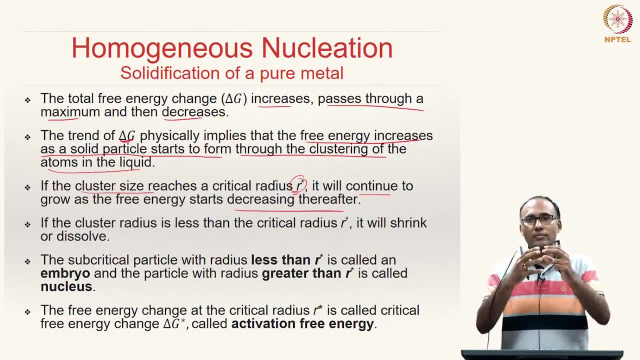 liquid state to solid state reaches a critical size called r star. that is when the nucleus continues to grow, because after r star the delta G starts decreasing. However, if the cluster radius- the cluster radius means the radius of this cluster of atoms which are trying to form a nucleus- is less than the critical radius, then what happens? 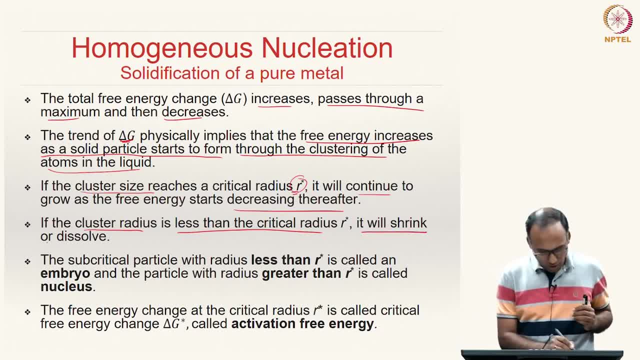 because it is not energetically favorable, then it will shrink or dissolve. It cannot have… It cannot be stable because energetically it is not favorable, because if it is less than r star, further increase will actually make it increase of free energy, which is not 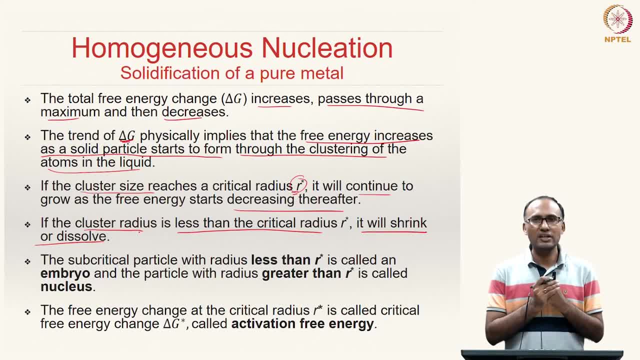 total free energy is increasing, which is not energetically favorable situation. So the subcritical particle with radius less than r star is called embryo. So that means if your particle size is less than r star, then it is embryo which will eventually dissolve. 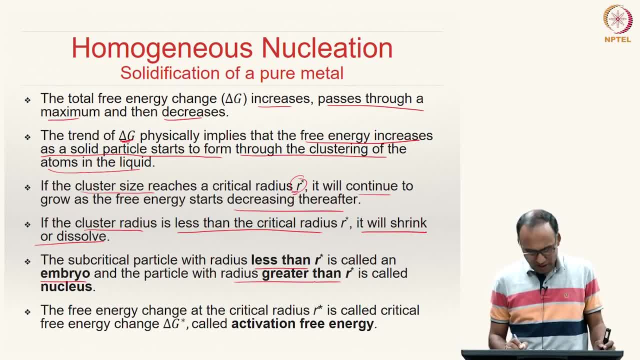 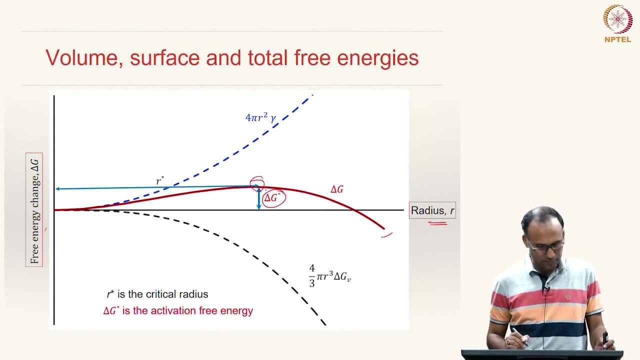 or shrink And the particles with radius greater than r star are called nucleus. So the free energy change at the critical radius r star, as we have seen here, at this critical radius the free energy change is delta G star. So the free energy change that corresponding to the 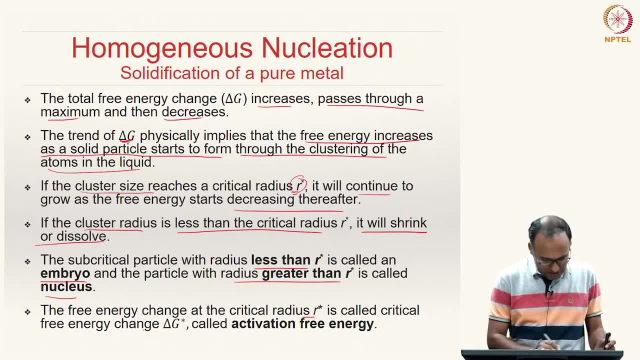 critical radius r star is what we call critical free energy change, delta G star, or it is also called activation free energy, and that is important, Right. So the activation free energy is the free energy change at the critical radius r star when the radius of the cluster… the radius of the cluster of atoms reaches your critical. 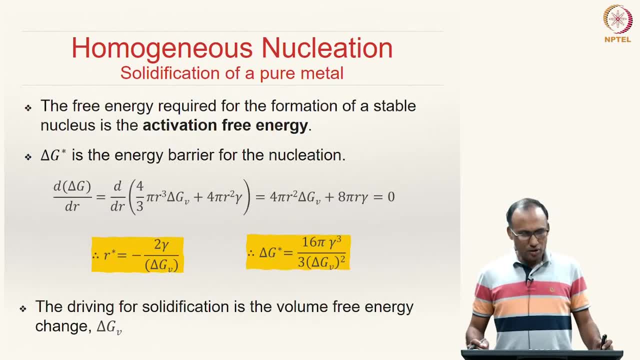 radius r star. Now, the free energy required for the formation of stable nucleus is what we call activation free energy. So this is the free energy change that is required in order to form a stable nucleus. Otherwise, if we have active nucleus, these are known as the activation free energy. 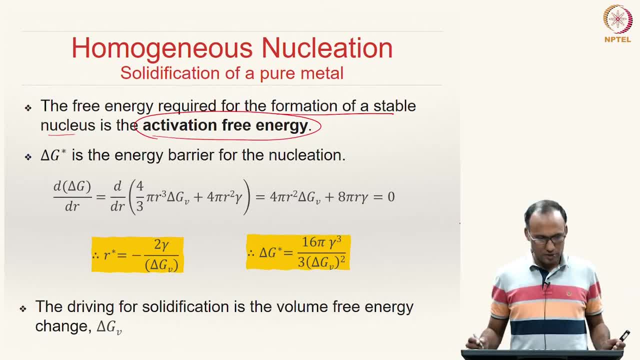 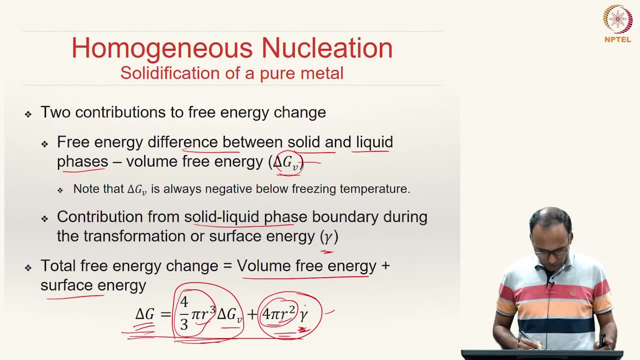 that nucleus will be unstable and then it will again dissolve. So the delta G star. so we know what is. we have seen what is G as a function of R. Now let us find out what is. so the delta G star corresponds to the maximum value of G delta. 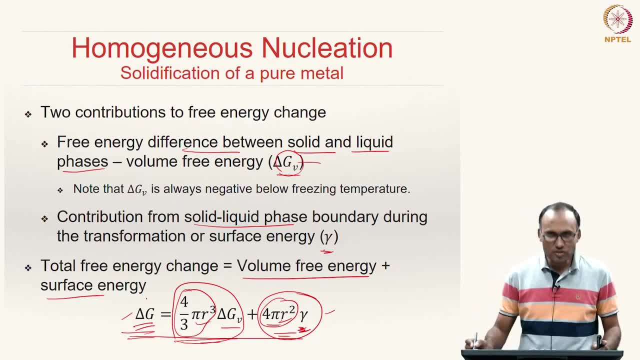 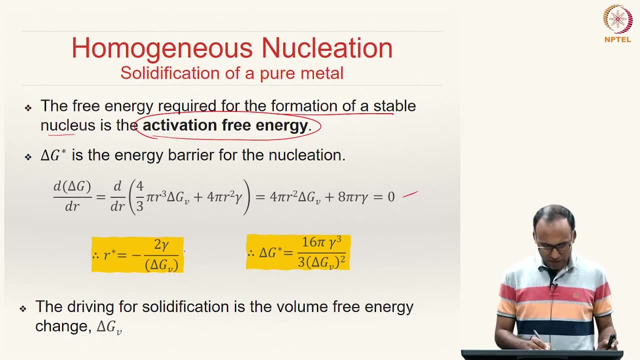 G as a function of R right. So we can find the derivative of this delta G with respect to R and then equate it to 0 in order to find the maximum value. and we do that, then we get R. star is equal to negative of 2 gamma by delta GV, where gamma is the surface energy. 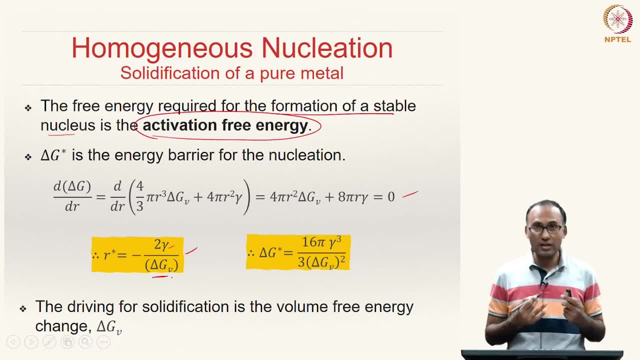 delta GV is our volume free energy, So it basically the radius. the critical radius depends on the surface energy and the volume free energy of the system. And what is the critical free energy change or the activation free energy is basically 16 pi gamma cube. 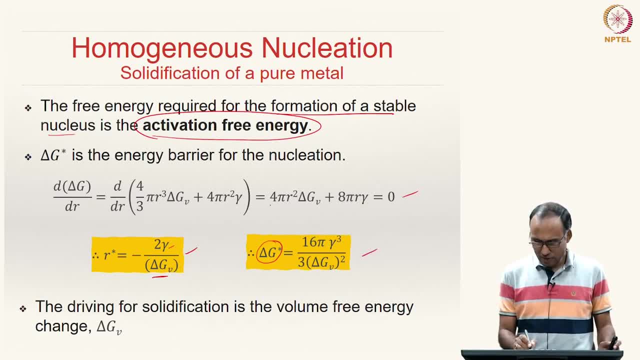 by 3 times delta GV whole square, as we can solve this equation to get the R star and then You solve this equation to get R star and then plug in this equation into the equation of delta. G is equal to 4 pi R square delta GV time plus 4 pi R square gamma plus 4. third, 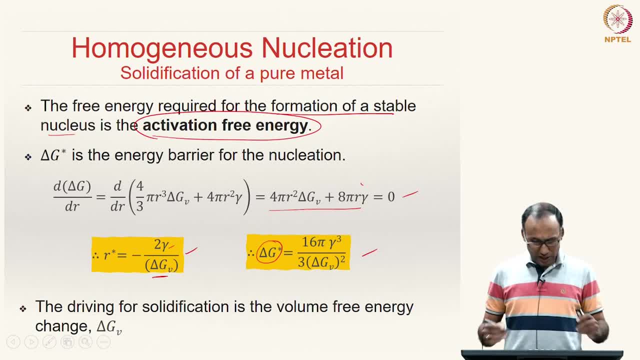 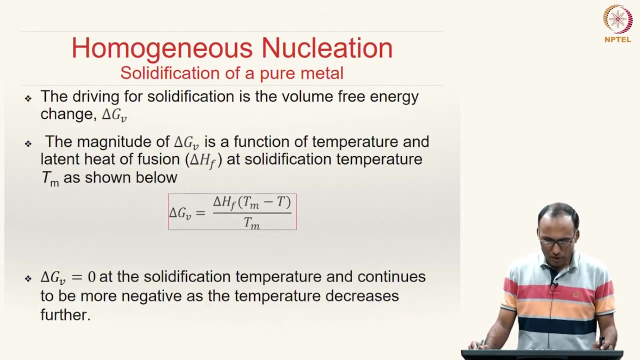 pi R cube delta GV, as we have seen before. So the driving force for the solidification is actually your volume free energy, delta GV, right? So if you have less activation free energy, then it is much easier for the formation of nucleus. So the magnitude of the delta GV: so, as we, the delta GV is our volume free energy. So 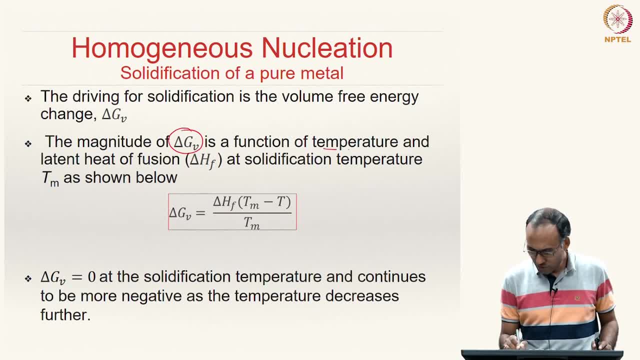 the magnitude of this volume free energy is a function of temperature and latent heat of fusion. What does this depend on? The magnitude of volume free energy? change in delta GV is our volume free energy. It depends on the temperature and the latent heat of fusion, which is defined by delta HF. So now I can replace my delta GV using 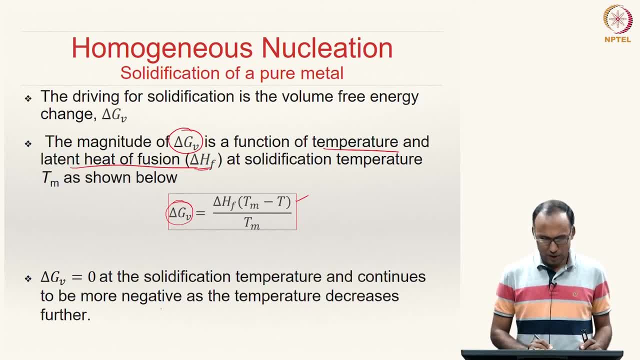 this expression the relation between delta GV and latent heat of fusion and temperature, where T, m is the solidification temperature or melting temperature, T is the temperature at which we are measuring, or we are actually trying to find out, what is volume free energy. So volume free energy is a function of temperature. So at the solidification temperature, right. 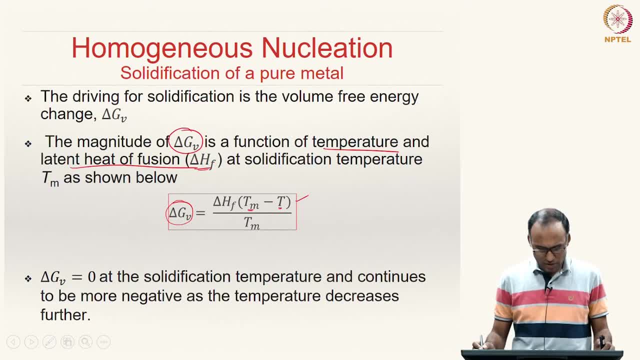 that means T, m equal to T, the delta GV becomes 0 and beyond that. So suppose, if you reduce T value below the solidification temperature, we know the delta HF is negative because its latent heat, heat of fusion, that means heat not supplied. But 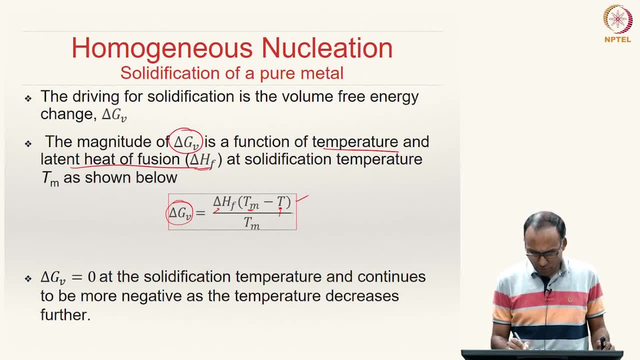 heat is given by the system and hence it is negative and hence it becomes more and more negative. right, As you are reducing, suppose let us say, this is our T m, and if you reduce your T, if you are making your T farther away from Tm, then this delta Gv becomes more, and 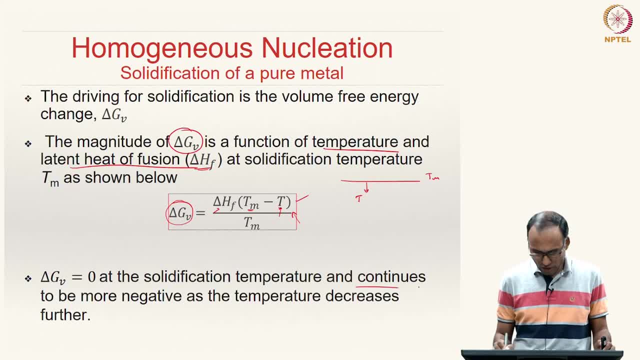 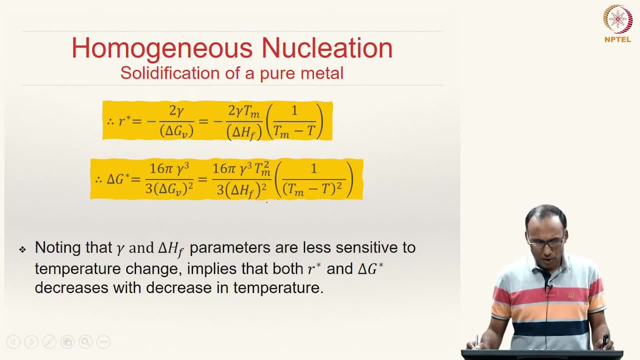 more negative. So at solidification temperature it is 0 and continues to be more negative as temperature decreases further. Temperature means this T. All right, So now we can write our r star and delta G star in terms of latent heat of. 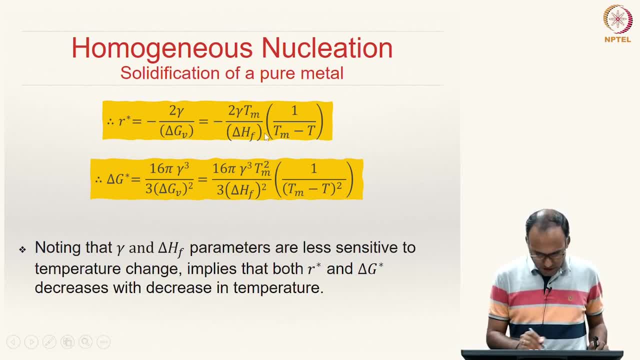 fusion and temperature And you can clearly see that so r star is a function of is written as function of gamma Tm, delta hf and the temperature Same is delta G star. And note that the quantity is the surface free energy, gamma and latent heat of fusion delta hf. 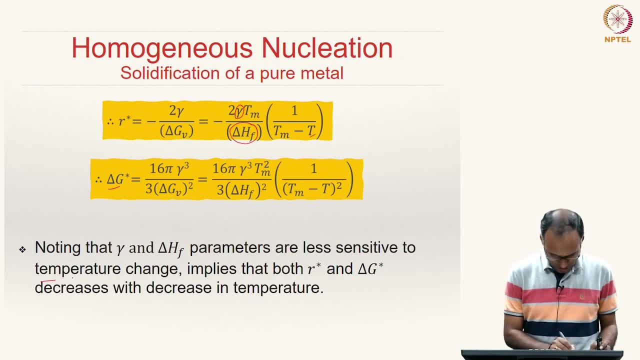 These two parameters are usually less sensitive to temperature change. They are sensitive but they are not very strong functions of temperature, So they are very less, much less sensitive to temperature change. It implies that your r star and delta G star. by looking at the way that this expression. 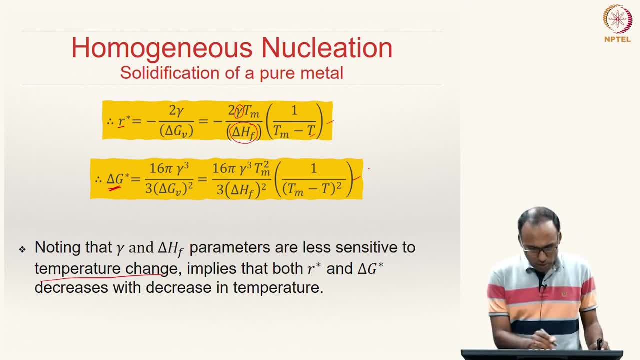 is. We can say that both r star and delta G star, of assuming gamma and delta hf are constants, they do not change with temperature. Then we can say that as you reduce your temperature, T r star and delta G star also reduces. right, because as you are reducing this number, this 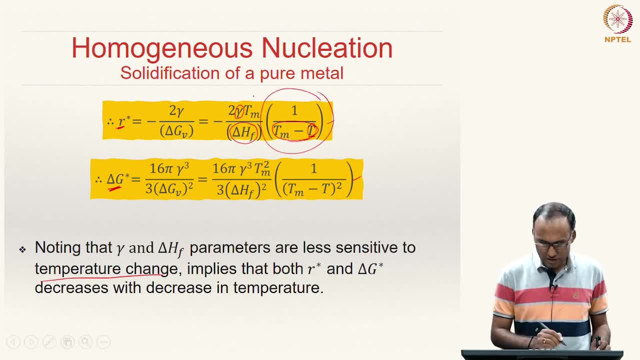 difference increases, as a result, fraction reduces and hence you will have lower value of r star. So if you would plot the r star and delta, sorry. delta G as a function of temperature. so in the expression where you have, delta G is equal to 4 third pi r square, delta G v plus 4 pi pi r cube, sorry. 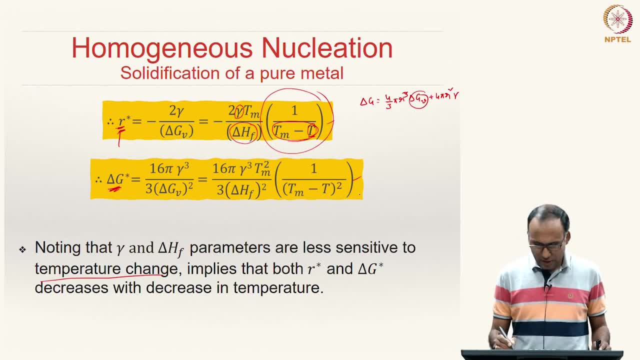 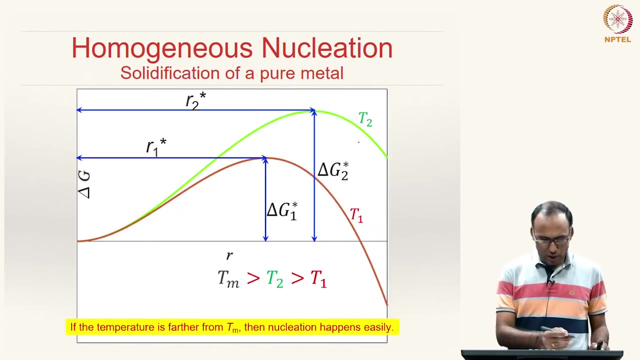 4 pi r square gamma. you replace delta G v with the expression that delta h f times T m minus T divided by T right. So, and then we can find the expression for delta G, and then we can plot the delta G as a function of r for different values of temperatures. 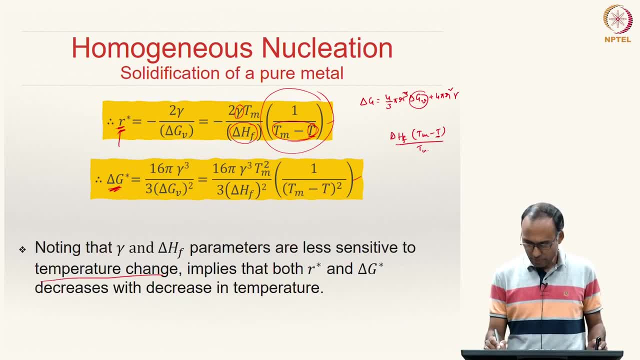 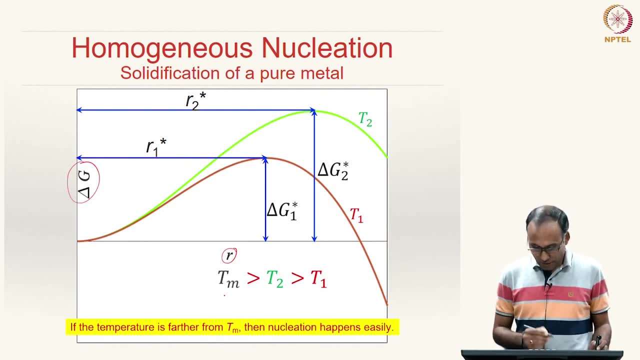 because here the delta G now can be written as a function of temperature- yeah, temperature, and then we would be able to plot delta G for different temperature values. So here I am plotting. so let us say T m is somewhere up here where your delta G v is 0. So T m? 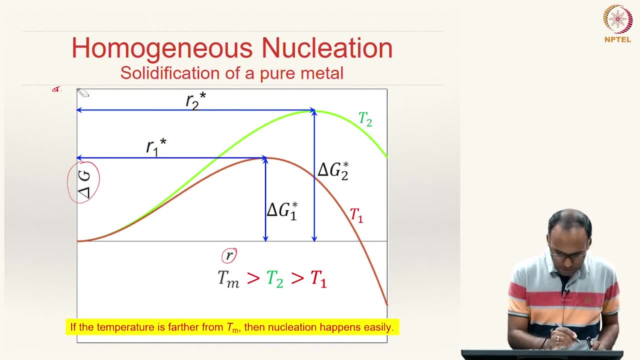 is somewhere up here. this is, let us say, this is my sorry, this is not temperature, I am sorry. this is delta G v. Now, if I am plotting delta G as a function of r at two different temperatures, where T 2 is greater than T 1.. 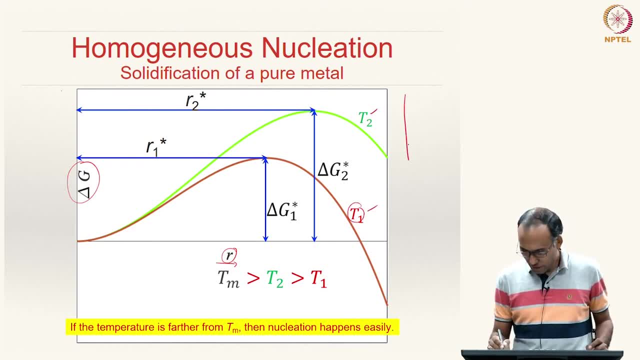 So T 1 is smaller. so, if you are on the T square, if this is my T m and that is, let us say, T 2 and that is my T 1.. So T 1 is smaller than T 2 and T 2 is smaller than T. 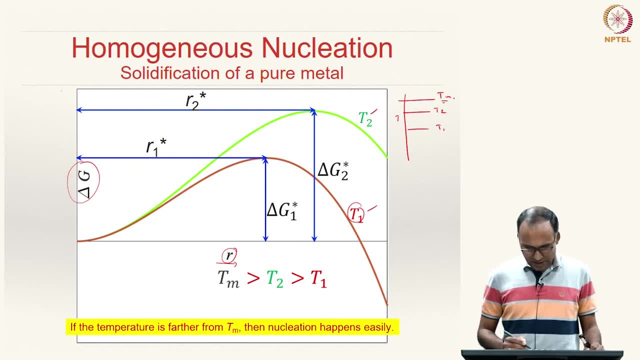 m right, Then we can clearly see, as you are reducing the temperature, your r star, r 1 star and r 2 star. so you can see that r 1 star is less than r 2 star and delta G 1 star. 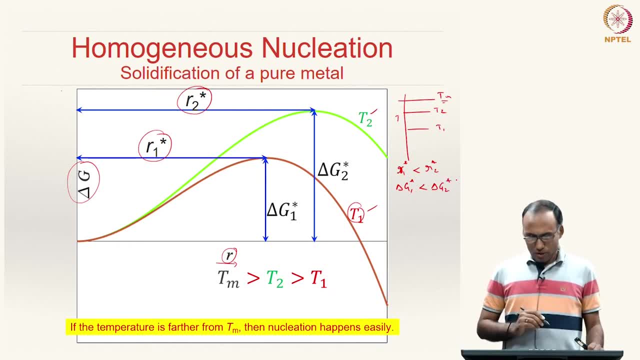 is less than r 2.. So delta G 1 star is less than r 2 star and delta G 1 star is less than delta G 2 star. So at lower temperatures it is much easier for the nucleation to happen. 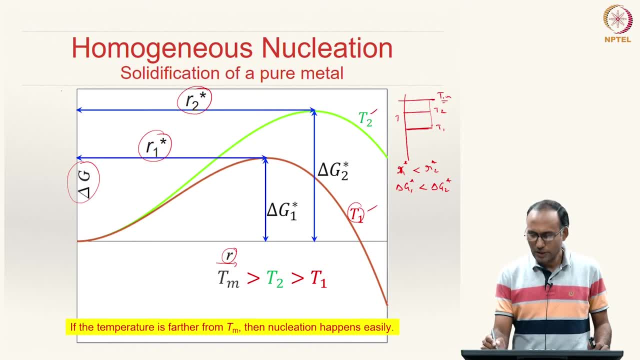 right. If your temperature is far away from that- the freezing temperature- then the radius- critical radius- is less and the activation free energy is also less And hence the solidification. so the nucleation happens more readily at temperatures farther from the solidification. 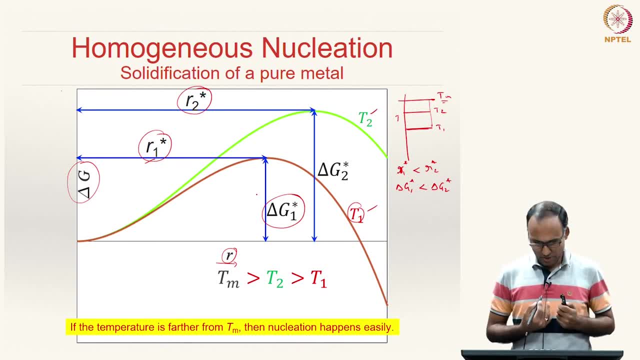 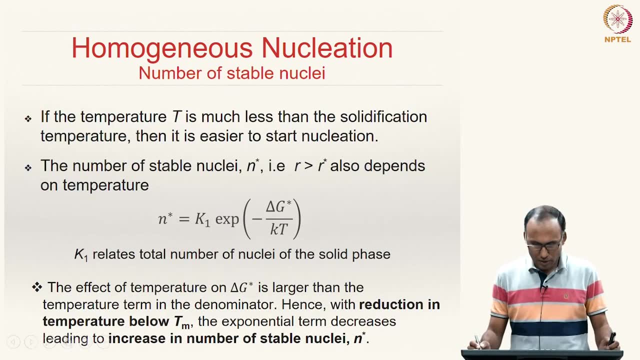 So that is why we have started at the solidification temperature or temperature for below the solidification temperatures. So if the temperature is farther from T m, the nucleation happens easily. So that is what we are trying to say. if the temperature is less than the solidification. 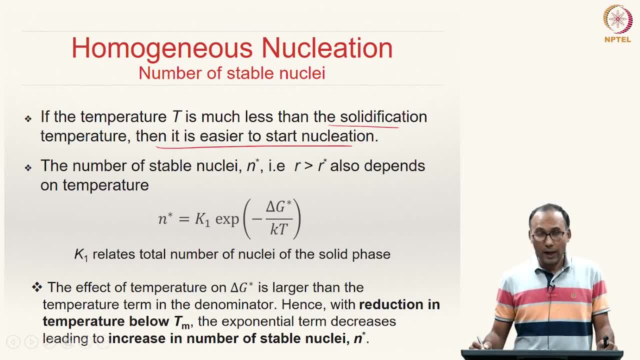 temperature, then it is easy to start nucleation. And so you are talking about, we have focus so far, our attention to the nucleation of one particle, but the number of, because we we are talking about homogenous nucleation, So the number of such stable nuclei n star. 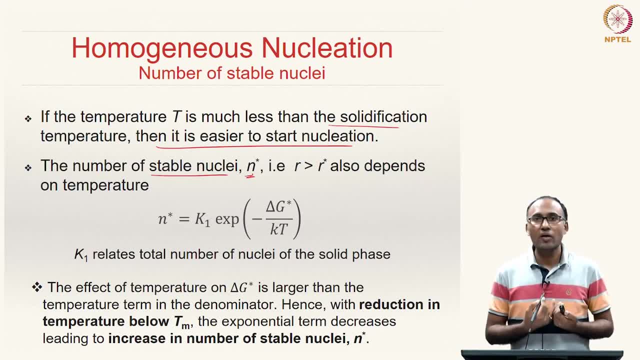 which is whenever, say we are saying stable nuclei, n star, that means for all these n star nuclei the radius is greater than r star. that also depends on temperature. So the n star can be expressed as a function of delta g star and the temperature right for given temperature. 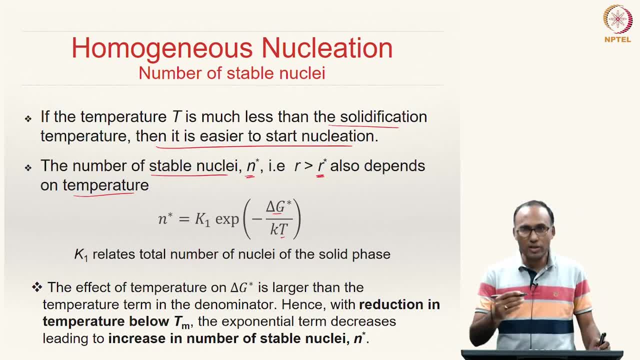 we know what is the delta g star and, as a result, as you are reducing your, So you can see that here n star, you know, the delta g star is also a function of temperature and t is also another factor. So this n star, as you know, with increase, with reduction in. 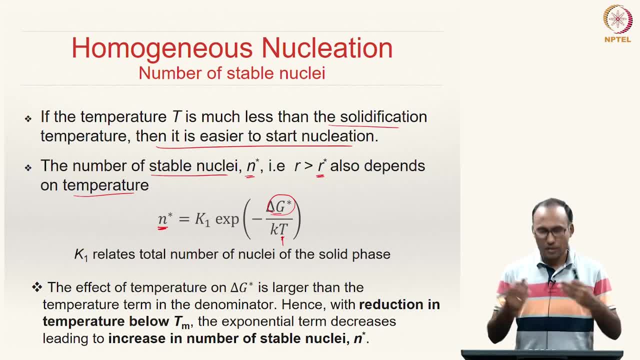 temperature, the delta g star reduces right So, but with reduction in. So this term, the, this term, The in the exponential has the effect of temperature on the numerator as well as on the denominator. right So, if you reduce the temperature, this entire quantity is increasing. if you keep, 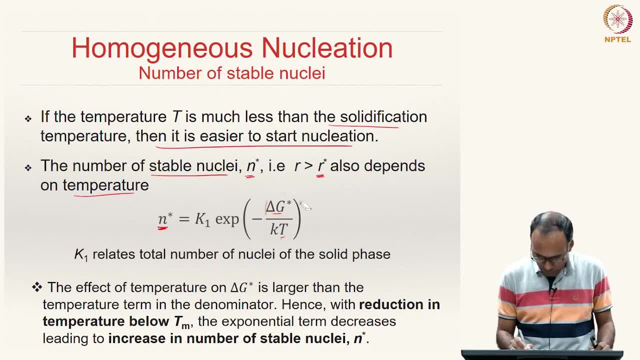 delta g star constant. right, So let us carefully look at it. So, if you are, let us say we are. we are saying that delta g star is constant, which is t is not normally, it is function of temperature. Let us, for the sake of sake of argument, let us say delta g star is constant. 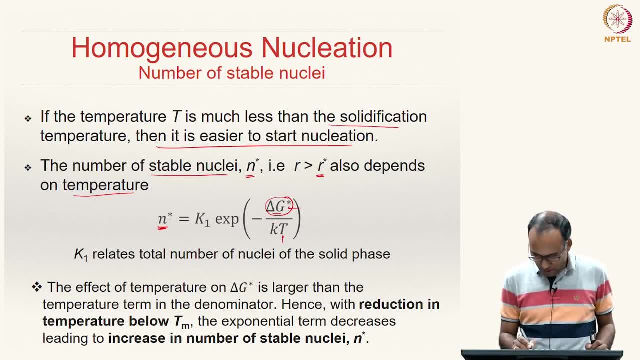 Then, as you reduce the temperature, this fraction increases. So as you reduce the temperature, the fraction increases. Now let us forget about the effect of temperature. Now we know that, as as you reduce temperature, the delta g star reduces, right? So now you have two. 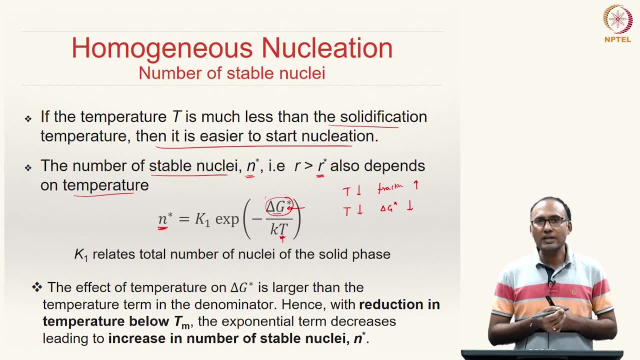 terms on the numerator, the numerator term with as an effect which is opposing the effect that is caused by the denominator term right, because the temperature also going to affect and delta g star is also a function of temperature. So the effect of temperature, however, is: 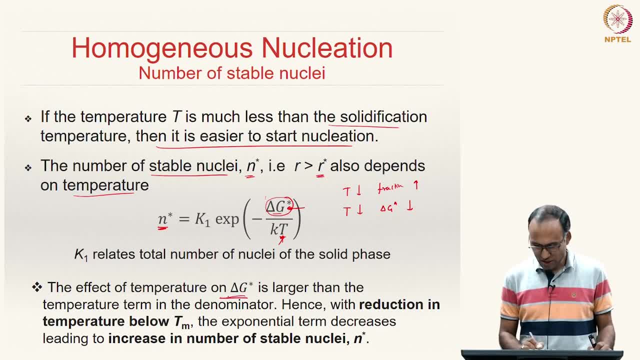 larger on delta g star. So the effect of temperature on delta g star is larger than the temperature term in the denominator. So with the reduction in temperature below T m there exponential term decreases. that means this term decreases, But it is a negative. there is a negative here and as a result the 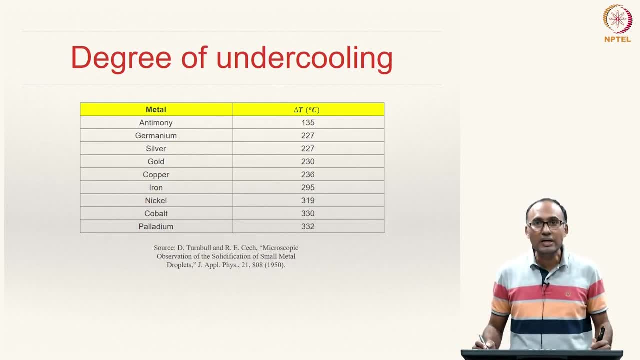 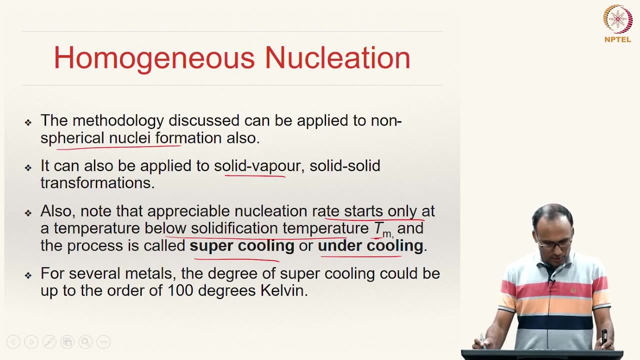 temperature from the solidification temperature is what we call degree of under cooling or degree of super cooling. all right, So for several metals the degree of super cooling could be of the order of 100 degrees Kelvin. for several metals, for homogeneous nucleation, if you would calculate So, the degree of super cooling would be around 300 degree Kelvin. 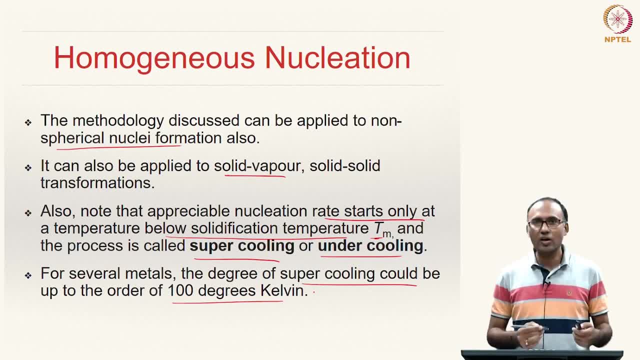 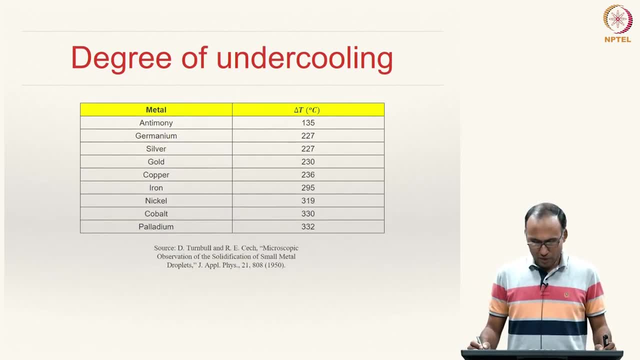 So we can see what is this. that delta T that we are talking about is the degree of super cooling. So this table here shows the degree of under cooling for several metals. for instance, if you take iron, So you need to for the nucleation rate to have an appreciable. 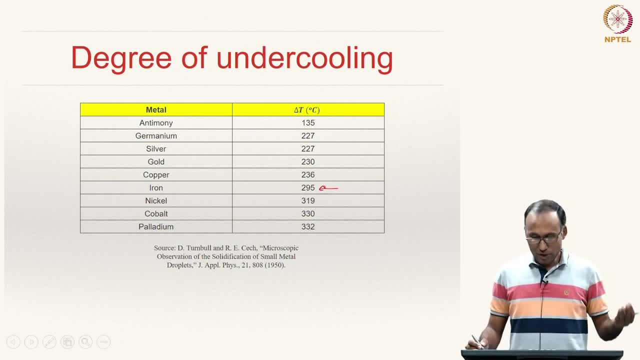 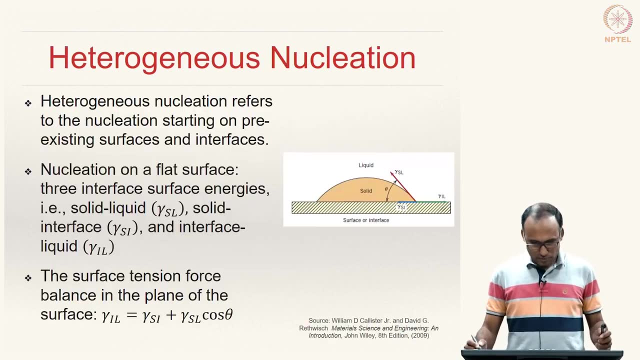 number. you need to under cool iron, pure iron, to almost 300 degree Kelvin or 300 degree Celsius, So it is few hundred degrees Celsius. 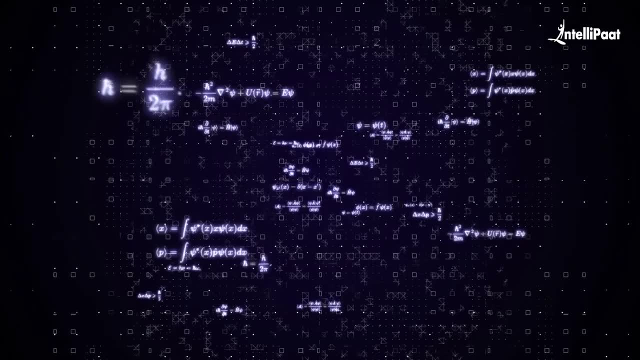 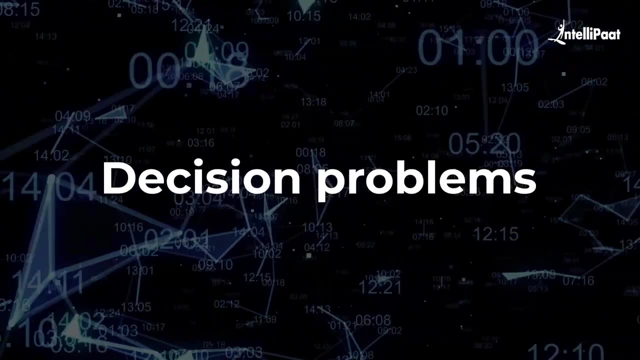 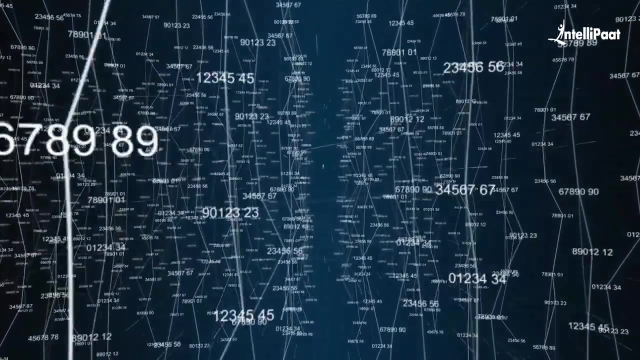 Hello everyone and welcome to today's session on NP problem by Intellipaat. NP is a set of decision problems that can be solved by a non-deterministic Turing machine in polynomial time. In this session we will talk about all the details of NP problem and its characteristics. 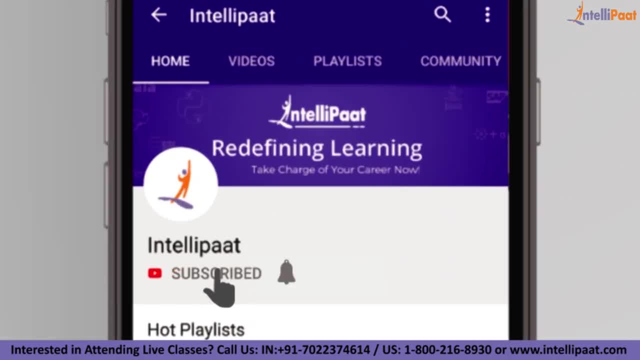 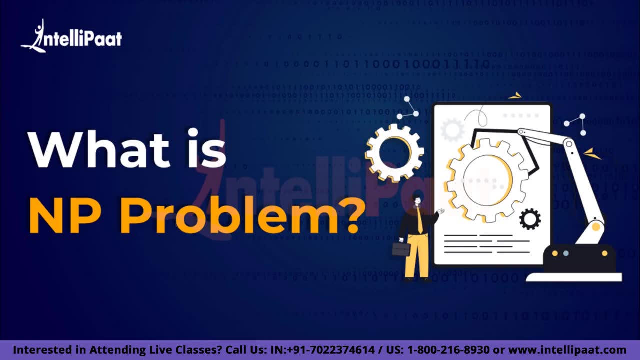 So, without further wait, let's start the session. But before we begin the session, make sure to subscribe to our channel and press the bell icon so that you'll never miss any update from us. Hello and welcome to yet another video by Intellipaat. In this video, I will be talking. 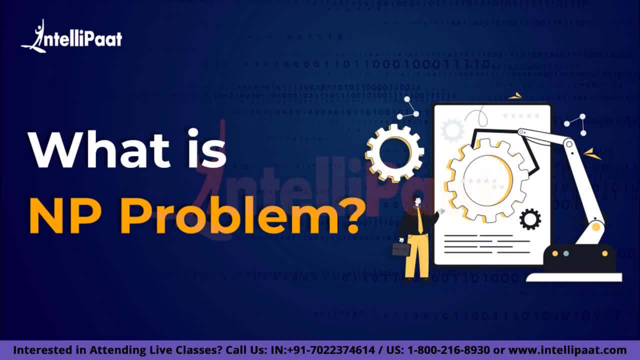 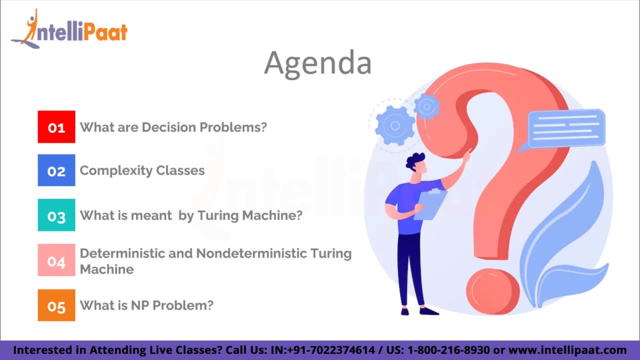 about the NP problem. By the end of this video, you will be able to know what are decision problems: complexity classes. what is meant by Turing machine, deterministic and non-deterministic Turing machine? what is NP problem? why are some NP problems hard to solve? some characteristics: 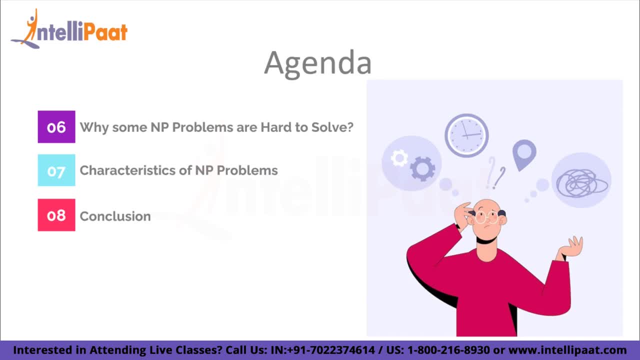 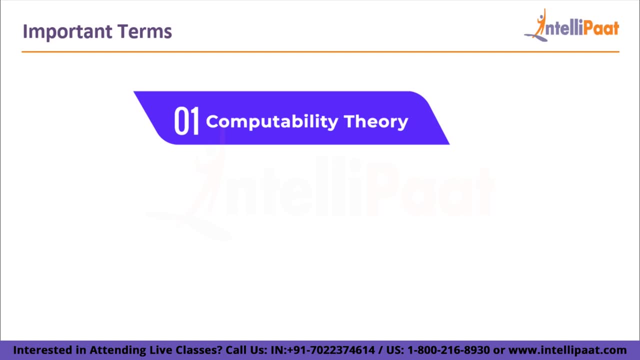 of NP problem and a simple conclusion. Now, before we move forward with today's agenda, let us take a look at some of the important terms. First, we have computability theory. Computability theory is a branch of mathematics that is concerned with the concept of an effective procedure, one that can be carried out by